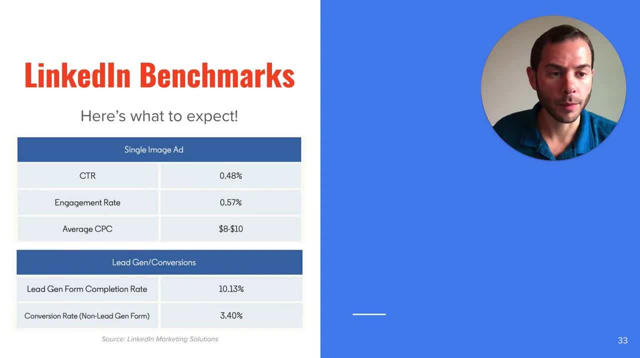 benchmarks that we see on the platform and these right here are published by LinkedIn, So you can see the average click-through rate is about 0.48%. Average CPC is between 8 to 10 bucks and I'd say that's for middle-range professionals in the US. When you go outside the US, 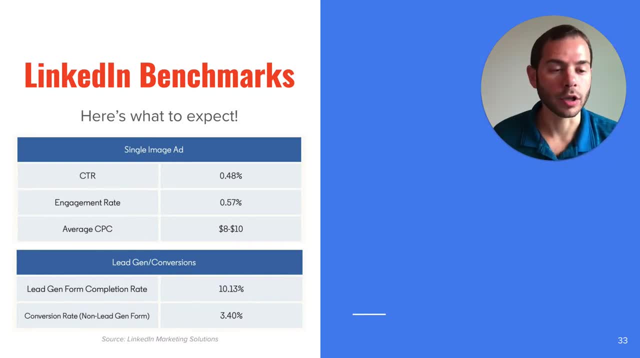 those numbers tend to be cheaper. and then if you target lower-level people, they tend to be cheaper. But also if you target higher-level people, such as like VPs, CXOs and owners, this number could be even higher for CPCs. So it's around. Because it is an auction, your average CPC is going to. 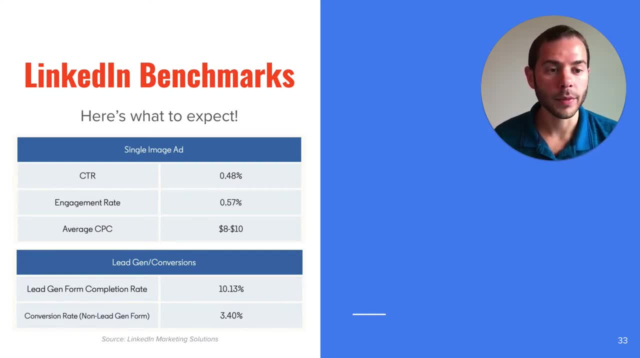 depend on how competitive the audience that you're bidding for is. If a lot of people are bidding for that same audience, often owners, More people are targeting owners, so owners tend to be more expensive, Whereas if you have a less competitive audience, your average CPC would be less because there's less 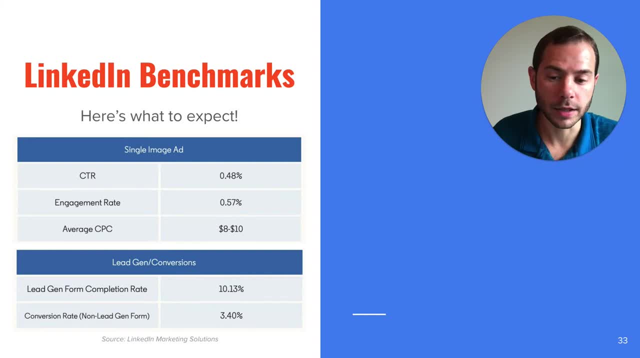 people bidding and they're bidding less on those people. So average CPC on LinkedIn does tend to be between 8 to 10 bucks. Within I'd say we are seeing a little bit higher. for middle-level people It might be 8 to 10 or 8 to 12 dollars in the US. Also, here are some conversion rates: Lead forms. 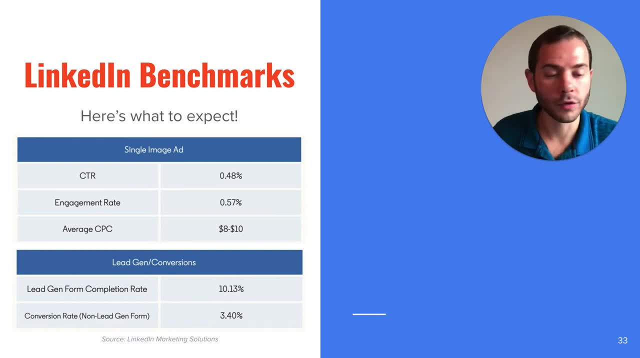 which is that little form that opens inside of LinkedIn. When somebody clicks on an ad, the average conversion rate for that is about 10%, And then for the conversion rate for non-lead forms. so when someone's clicking through an ad To go to a landing page to perform some action there, usually submit a form on that page or register for. 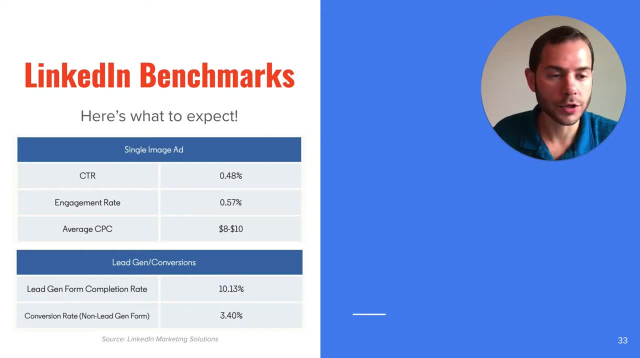 something. that conversion rate is about 3.4%. So all these numbers are important to know because these will calculate what your cost per action is, or cost per acquisition, and then these numbers can help calculate your funnel. So kind of what this comes down to is with an average CPC of about 8 to 10 bucks and then average lead. 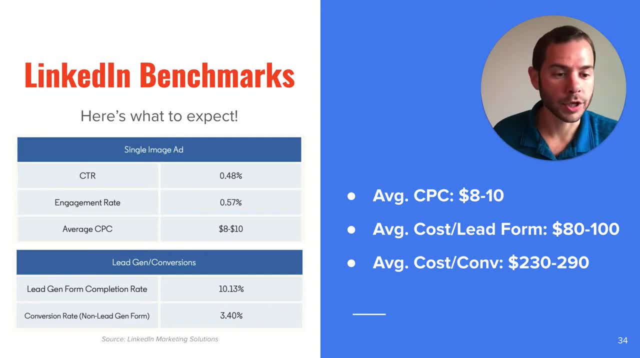 form completion rate of about 10%. LinkedIn's publishing here that the average cost per lead form is about 80 to 100 bucks in the US And then average cost per conversion- usually a form on a landing page- is about 230 to 290 dollars in the US. 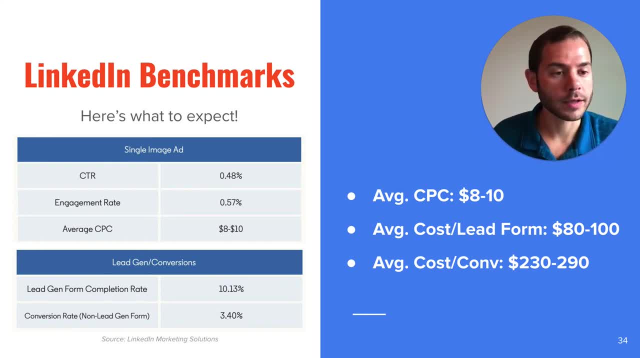 With our optimizations, we can usually get that significantly better than that, but it is interesting to see how much better lead forms can be for lead capture versus cost per conversion. It all depends on what your business needs to do and what your campaign needs to do, but these are some good numbers to know. 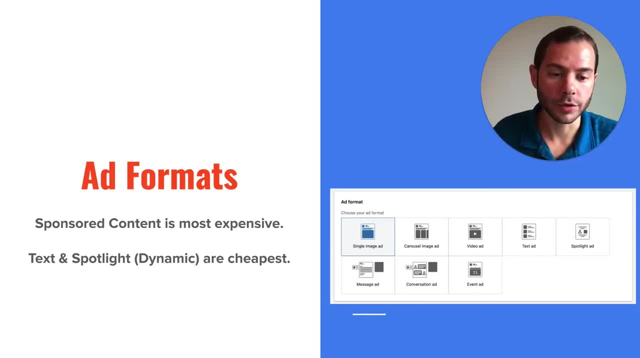 So first thing to talk about is ad formats. So this is kind of where cost starts coming into play. Sponsored content, ads in the newsfeed are the most expensive. So sponsored content and ads in the newsfeed, those can be single image ads, those can be carousel ads and those can be video ads. So the first three that you see in this graphic. 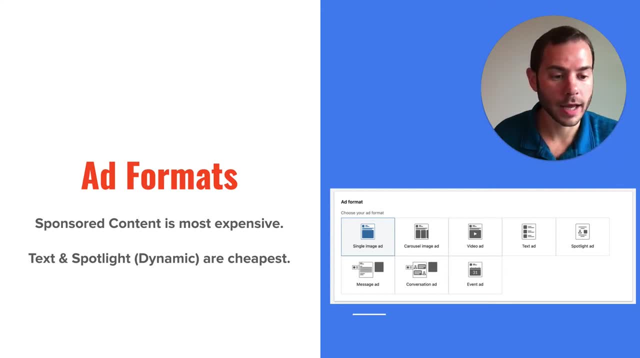 here. those are all sponsored content ads. After that you see text ads and spotlight ads. Spotlight is also called dynamic. Those two tend to be the cheapest. So most advertisers, most people on LinkedIn, they are using sponsored content. so it's partially because it's the most competitive. 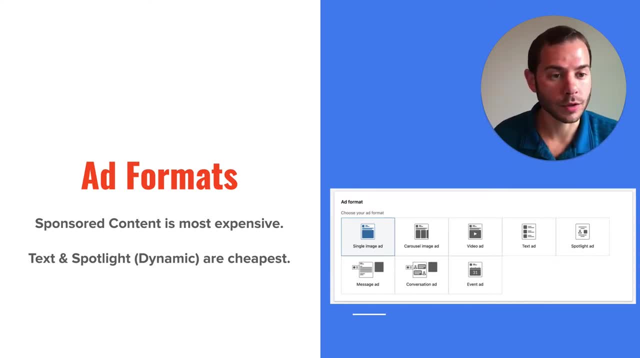 The most people are bidding For that same space, So that's why those ad units are the most expensive, Whereas text and dynamic less people are using those, and those clicks tend to be a lot cheaper. So if you're starting with sponsored content, it is a good place to start. 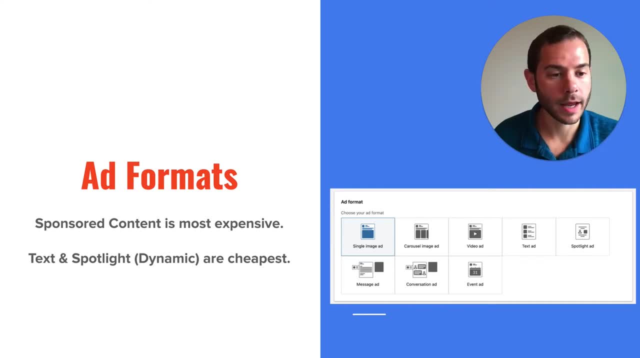 because it's a very high quality ad unit. You can have an image, a lot of text in the headline Text ads and dynamic ads are much smaller ad units and they only appear on desktop, So there's less information you can put in there. Often we'll start. 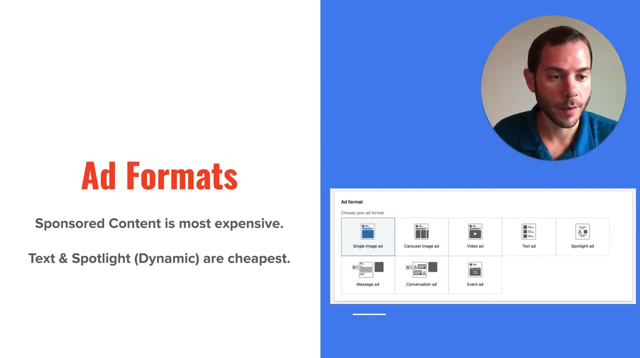 with sponsored content and then move on to text and dynamic. Once sponsored content is in the newsfeed, you can start with sponsored content and then move on to text and dynamic. Once sponsored content is in the newsfeed, You can start with sponsored content and then move on to text and dynamic. Sometimes we'll start 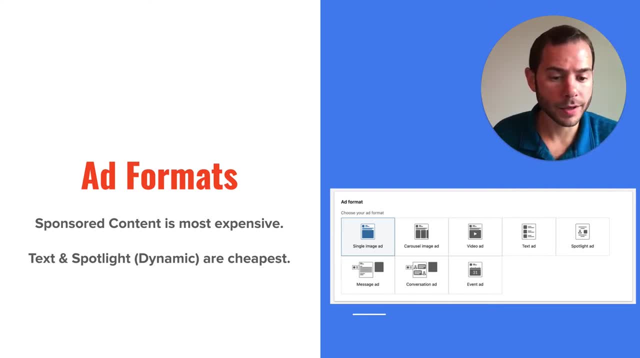 with sponsored content and then move on to text and dynamic. Sometimes we'll start with sponsored content and then move on to text and dynamic, But it all depends on the needs of the campaign. Messaged in conversation ads. those can be even more expensive because you're 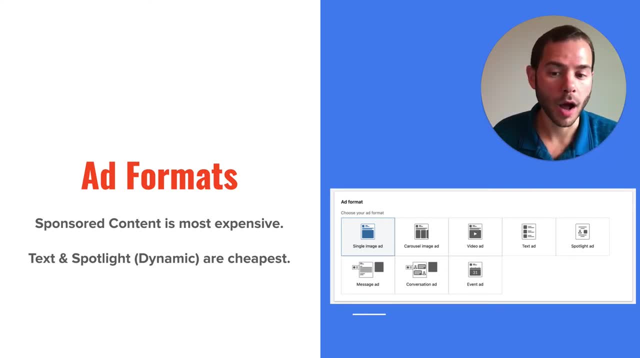 paying for every send, So it just depends on how- how much- your message resonates with the target audience. We often find that special invites or job recruiting ads can work very well as messaging conversational ads, But if your audience isn't clicking, It's an opting in. 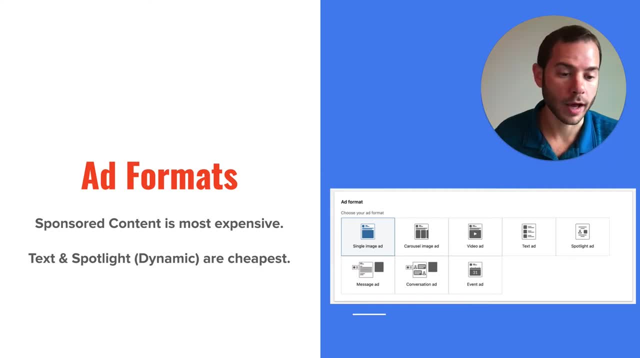 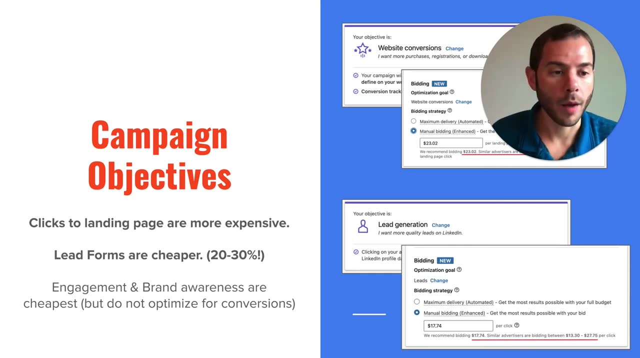 you can have a very high, the highest cost using those ads. Next is campaign objectives. So, depending on the objective that you choose for your campaign, that will also determine costs of how much you're paying per click and per impression. So it depends on the objective that you choose. 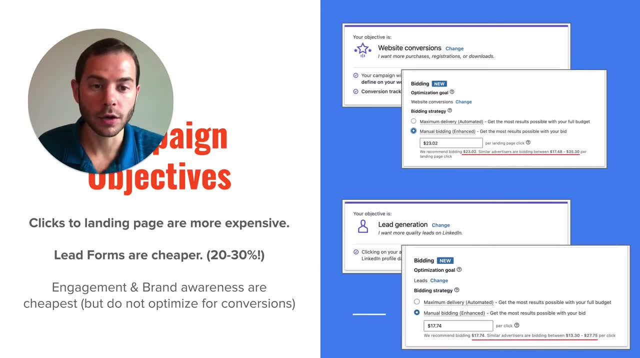 What's really interesting to see is that when you have a website visit or a website conversions campaign, any objective that sends people to a landing page and off the LinkedIn platform, those are the most expensive objectives. And when you think about it, if LinkedIn is losing traffic, you know people are clicking. 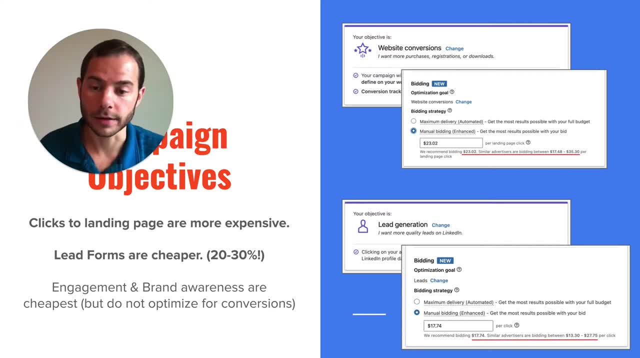 off their platform, they have less of an opportunity to serve that person- ads- So it kind of makes sense that those are going to be more expensive. You have to pay more to get that because LinkedIn knows you're losing some traffic, Whereas with lead forms they actually tend to be cheaper because people are clicking. 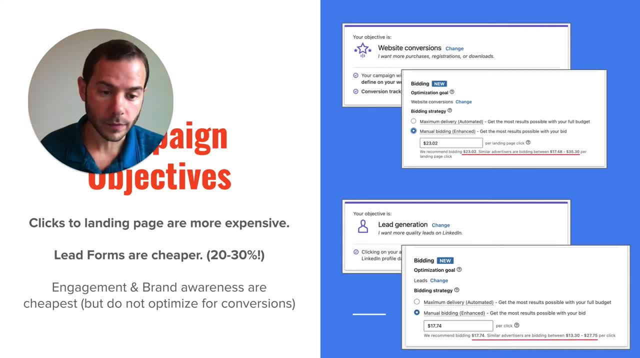 on the ad submitting that lead form on LinkedIn. So in LinkedIn's eyes that person staying on the platform, they have an opportunity to see more ads. use the platform more So it's more valuable to LinkedIn, So they give you a discount for using that. 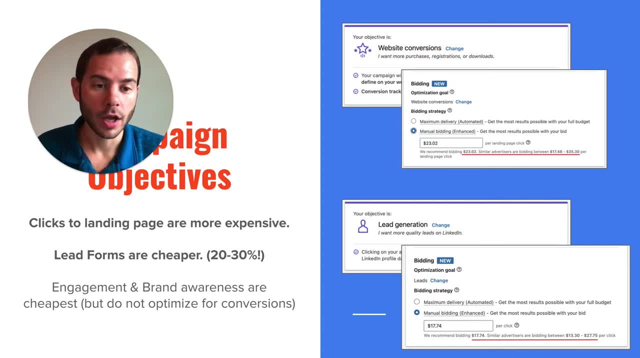 And what's really interesting is, if you pop in some numbers, You can go to the bidding section. I have two identical audiences here and I'm looking at the manual bidding ranges that they're suggesting For the top one here. this is website conversions. 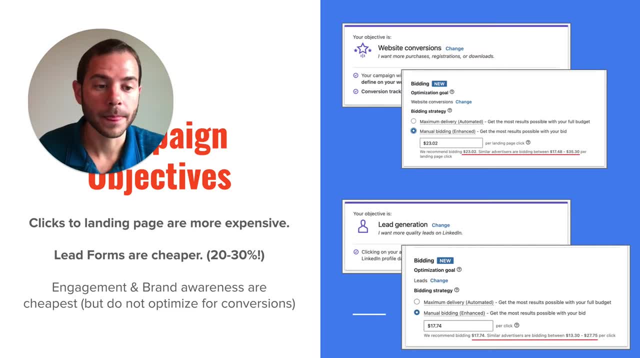 So when this would be when someone's clicking on an ad to go off the platform and LinkedIn's telling us the average bid is 23 bucks and the average range is 17 to 35. But if I switch that to lead generation and use the exact same audience and exact same? 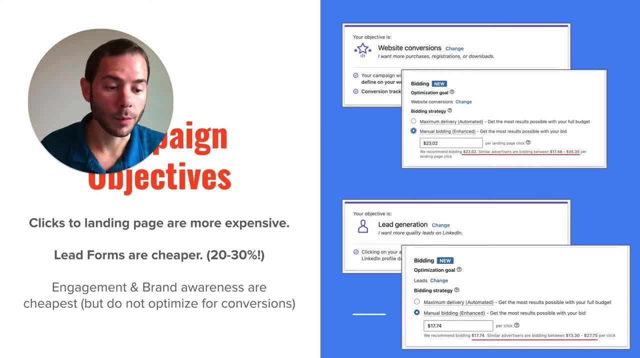 ad type. LinkedIn's telling me the average is 17 bucks or between 13 to 27.. So that's significantly cheaper- 20 to 30% cheaper. So that's interesting to know. If lead forms work for you, that could be a good way to improve your costs. 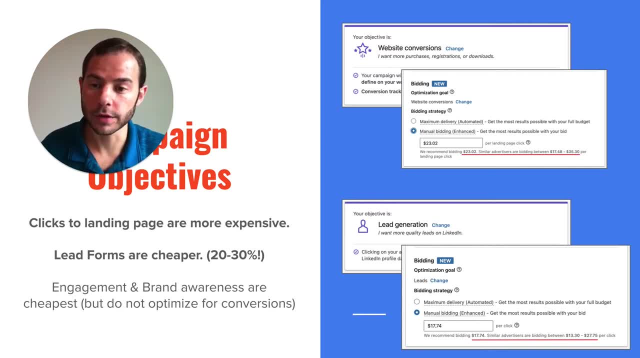 And then, lastly, engagement and brand awareness objectives are even cheaper than these two objectives here that I've mentioned, but they don't optimize for conversions. So if you have a campaign that's just blown it out of the water has an extremely high 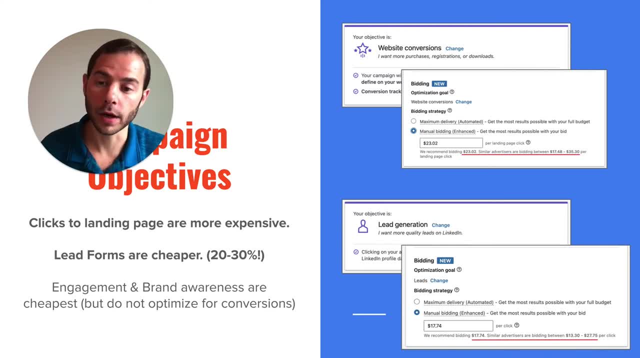 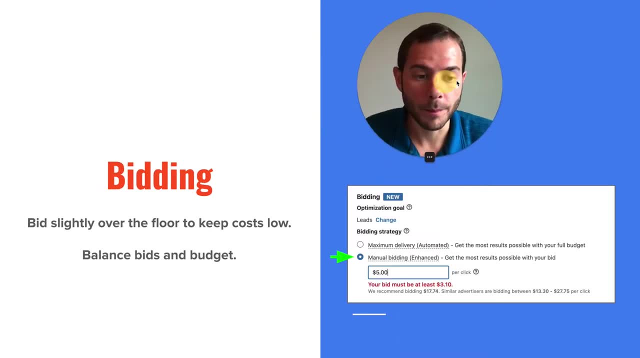 click through rate has an extremely high conversion rate, then you might want to consider testing out and experimenting with engagement and brand awareness. Next, here is around bidding. So by default, the campaign manager will automatically select automated here the first option. but 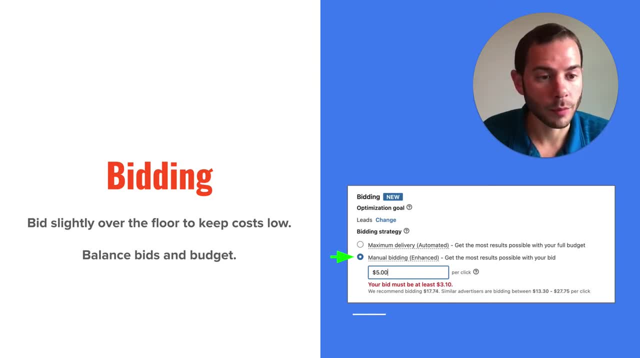 we don't see. most people usually want to start with that, Usually want to start with manual bidding, because when you do automate it, you kind of just turn it over to LinkedIn and say: here's my budget. Go ahead and spend as much as possible. 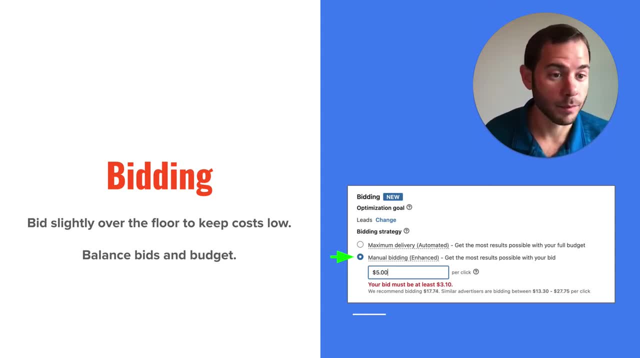 You can see it's also called maximum delivery. So you're telling LinkedIn: maximize my spend, spend all my budget. And LinkedIn does have a lot of very expensive people out there, So it's going to kind of go out there and advertise everything. So you're telling LinkedIn: maximize my spend, spend all my budget. And LinkedIn does have a lot of very expensive people out there. So you're telling LinkedIn: maximize my spend, spend all my budget. So you're telling LinkedIn: maximize my spend, spend all my budget. 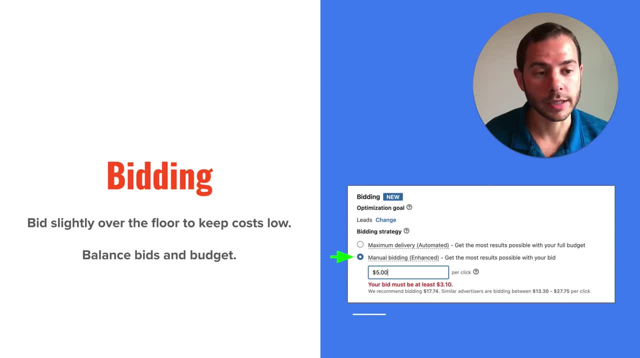 Including the very expensive people who you might not necessarily want or need to target because there's cheaper ones available. So most people do start with the manual bidding. We recommend starting with manual bidding, So flip it over to manual bidding here in the bidding section and then LinkedIn is. 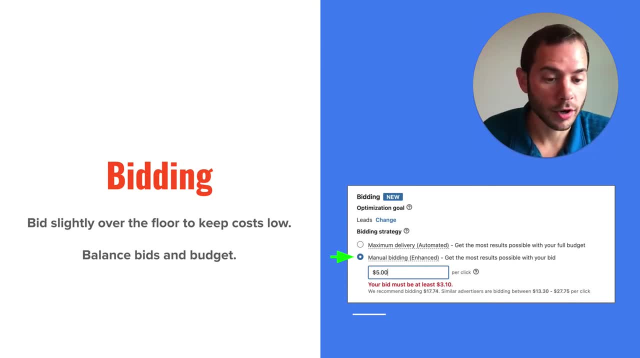 going to tell you some averages Here. you can see, for this audience the average is about 17 bucks, but they're telling us the range is like 13 to 27, and this is the. this is in the whole audience on LinkedIn. 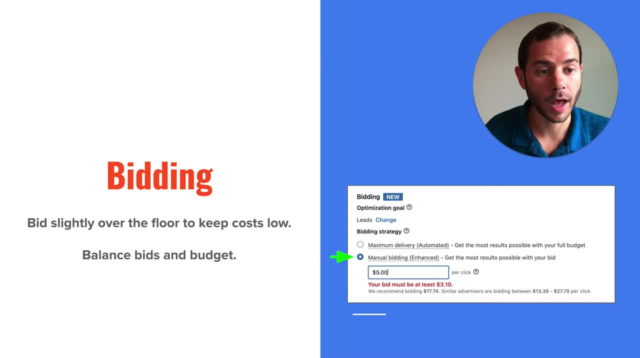 Now, keep in mind, LinkedIn is a big platform. There's a lot of very big companies and big companies, big advertisers, that advertise on there with very big budgets. So those are the ones who are spending- you know, spending- amounts in this range And we've managed many campaigns that are 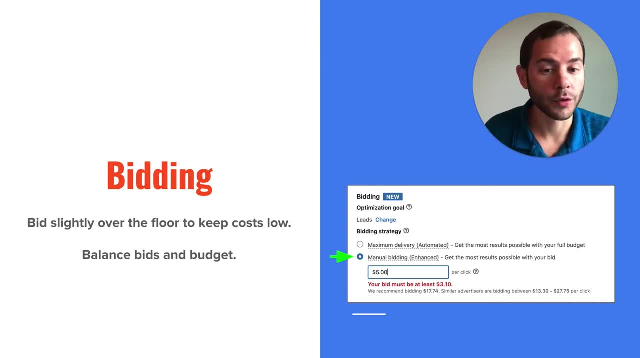 actively bidding and spending in that range. But for the average advertiser or if you're just getting started, we recommend you start bidding manual and you can even LinkedIn's going to suggest a recommended bid that they're going to start by popping in there. We recommend swapping. 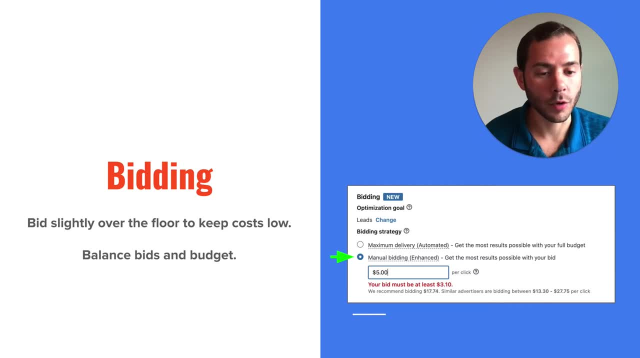 out that number and bidding. start by bidding as put in the lowest number possible. I'll like usually throw a one into this input and just see what LinkedIn tells me is the real floor for this audience. So if you put a one in here, LinkedIn is going to say: you know your bid must be at least. 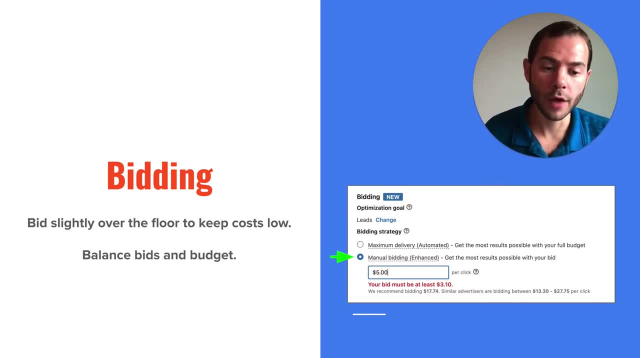 $3.10.. And that's the absolute minimum. If I bid the absolute minimum- you know I'm the lowest bid going into the auction- It's likely that I'm not going to get too many impressions. So it kind of depends on what your overall budget is for the campaign how fast you're looking to get impressions. 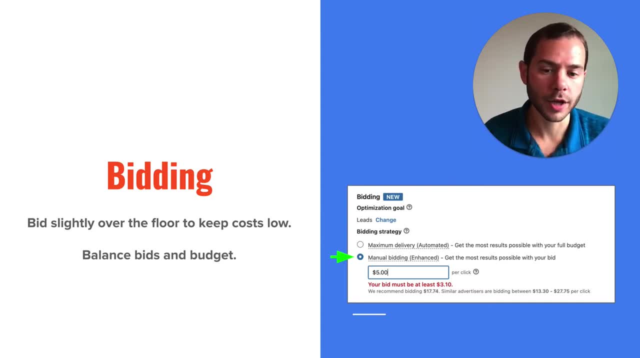 and clicks and conversions coming in. So usually what we'll do for the average campaign is start this about: we'll either start this with a minimum bid, or we'll start this with a minimum bid. We'll start this about 20% over the actual floor here, or we'll, you know, kind of take half of what. 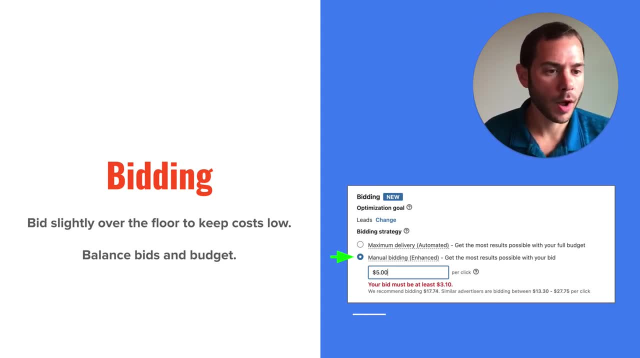 that lower range is somewhere in there. You know, if I know my audience tends to be more entry-level people versus more senior level people, then I'll kind of use that in my analysis of what to put in here. So if it told me the floor is about three bucks, I might start with five. I might start with. 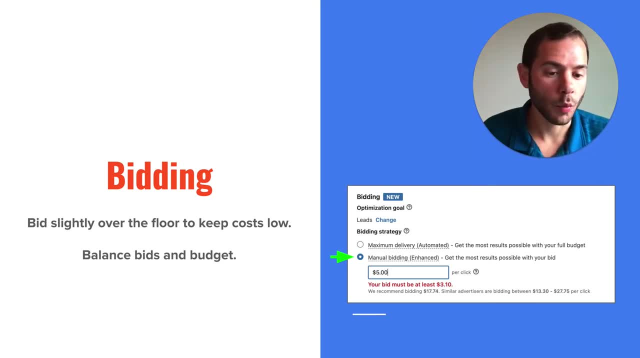 six and then see how that performs. So once you set your bid, you'll then want to keep an eye on your campaign and keep an eye on your impressions. If you see that you're just not getting many impressions at all, then you'll need to turn that up a little bit so that you make sure that you're. 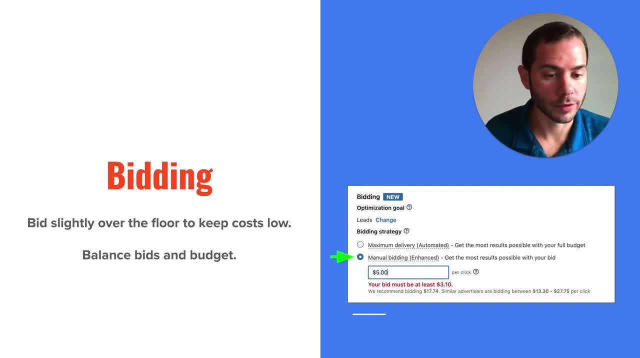 winning more auctions and getting more impressions and your campaign is getting served. The time to use automated bidding is when your CTR is really high and your budget is really high, So automated bidding is actually a. it's a CPM bid, so you're paying for every impression. The nice thing about. 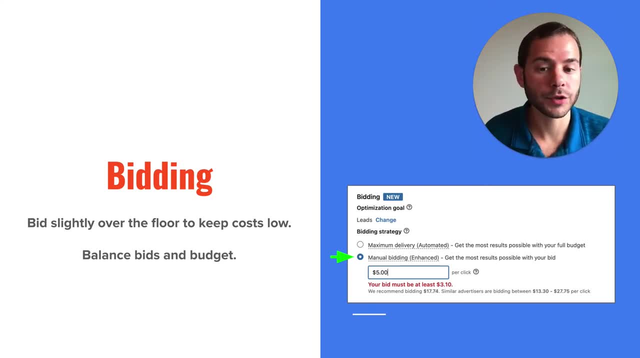 enhanced bidding. manual bidding here is that you're paying for every click. So if your ads have a lower click-through rate, you know. if you're doing some initial testing, you don't know what's going to get a good high click-through rate first. usually you want to start with manual bidding. 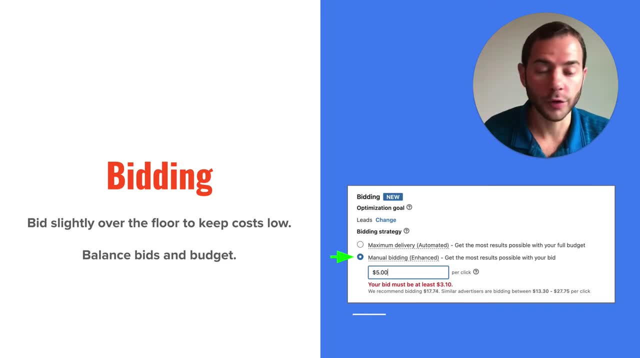 because you're only going to pay when people click. Once you've figured out what's the best creative, what's the best audience for you, and if you are getting a very high click-through rate- of over 1%- and your budget is very high, then that's when you can switch to automated bidding. 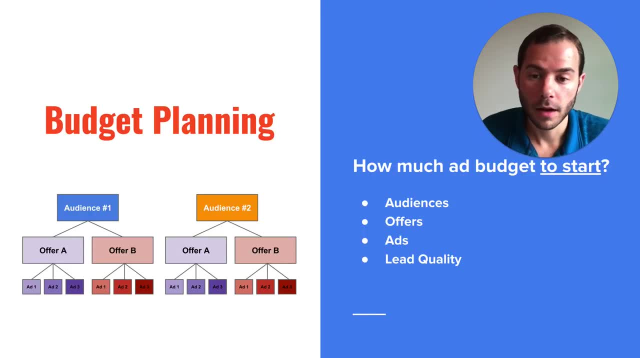 and get better results using that. All right. so then the next question is: how much budget do I need to start? So this kind of depends on how many clicks you're going to get If you're going to use the right audience you want to advertise to, how many different offers you want to use. 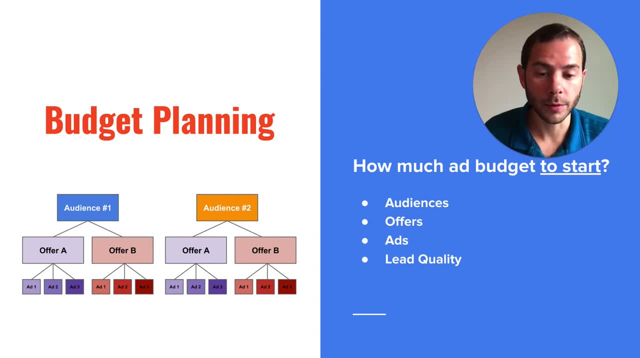 and then how many different ads. So you know, there's lots of different variables here and you can see that kind of standard campaign structure or an example of a campaign structure here on the left. We have two audiences here, we have two offers and then we have a couple. 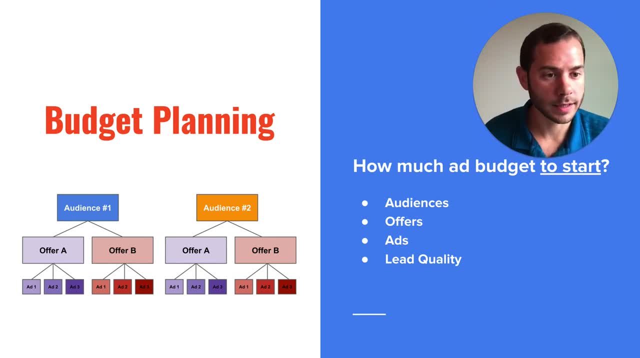 different ads below each of them. This is kind of a simple testing setup. You kind of you'd want to start with at least this so you can have some split tests, So you can split test your audience, you can split test your offers and then, of course, you can split test your ads below that. 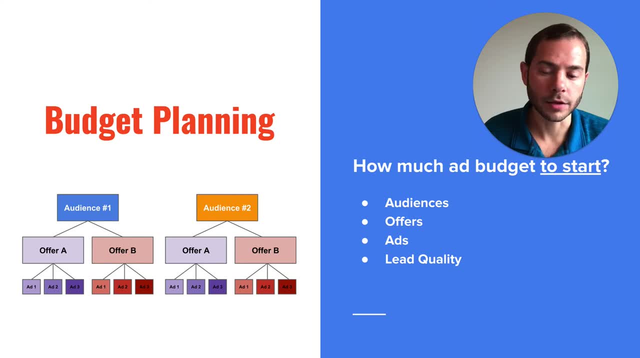 We usually see to cover all these different combinations. you know it's usually about 3,000 in the first month or so. If your budget is, if your monthly budget is less than that, you'll need more time to get that data in Again, because clicks on LinkedIn can be more expensive. 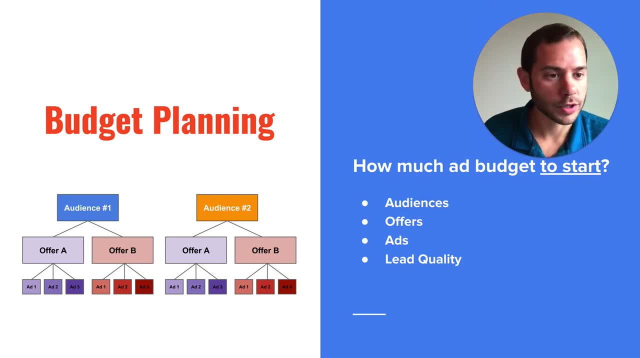 you know, if an ad only gets two or three clicks, then that's not going to really tell you anything because you need to have enough data, enough clicks, to be statistically significant. So usually we see the minimum budgets on LinkedIn, to get started, tend to be a little bit higher than. 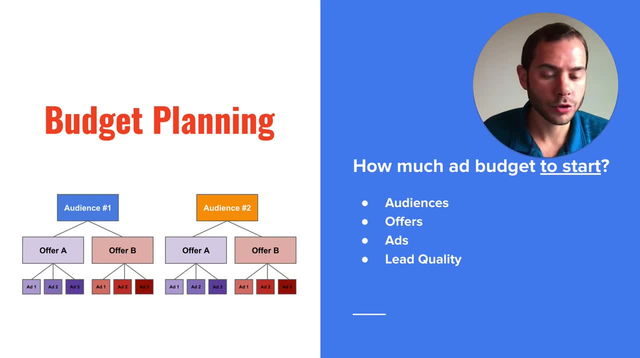 say Facebook or other platforms. You also need a certain number of leads or conversions coming into your funnel so that you can actually evaluate that lead quality Again. if you're only getting, you know, one, two, three leads, that's not going to really tell you anything. You might just have a fluke. 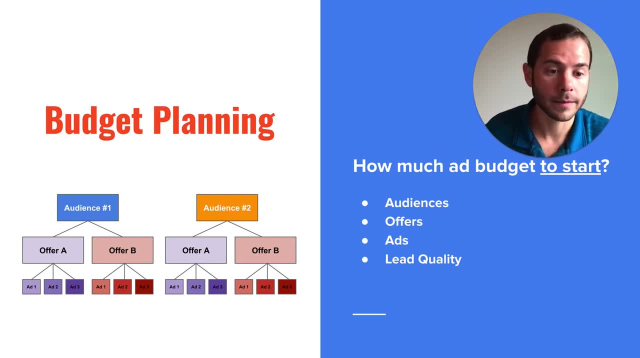 of a couple good leads or you might just have a fluke of a couple bad leads, So you'll need to have a significant number to make some decisions there. So, like I said, most campaigns and most offers need to start around 3,000 for the first month for campaign and lead evaluation to be able. 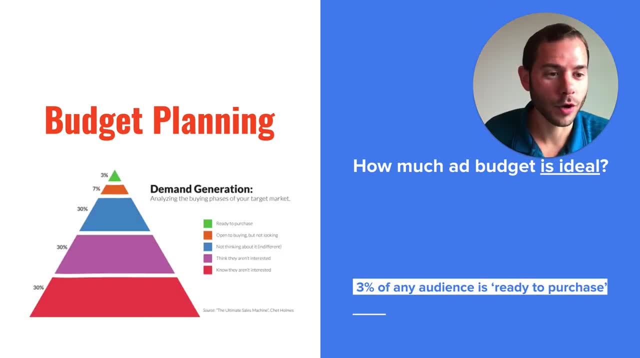 to get enough data to make those decisions All right, And then, once you're past the testing phase, how much budget is ideal? I'd say the first, the most important thing to think about when I talk about this is: this chart here on the left is very interesting because it shows: 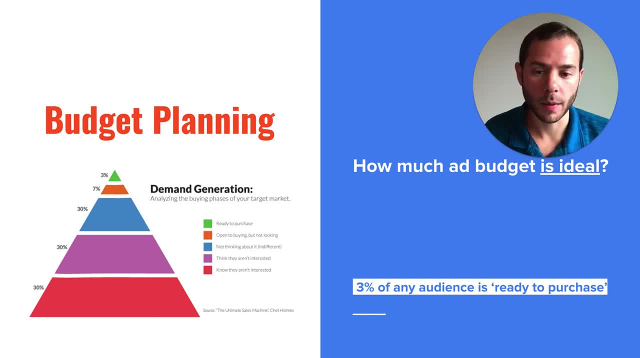 you. this is the average of you know your average market up there, how people fall into different categories In every audience out there. there are certain people who are, you know, actively looking for a solution and, you know, considering buying one. There are people who know it's. 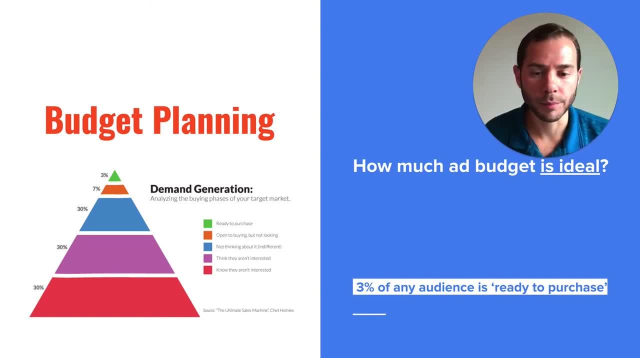 something that they're going to be thinking about in the next few months, but maybe they're not actively looking at prices or actively evaluating systems right now. And then you have a lot of other people who maybe are aware of it, but it's not their job, or you know. 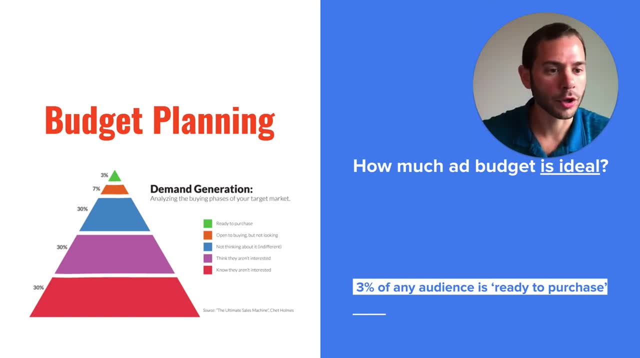 they're not. they know this might be in two to three months down the road. they're looking to make that decision. And then you'll have at the bottom level here, people who have no idea about this problem. They have no idea that there's a solution out there. So this chart kind of shows. 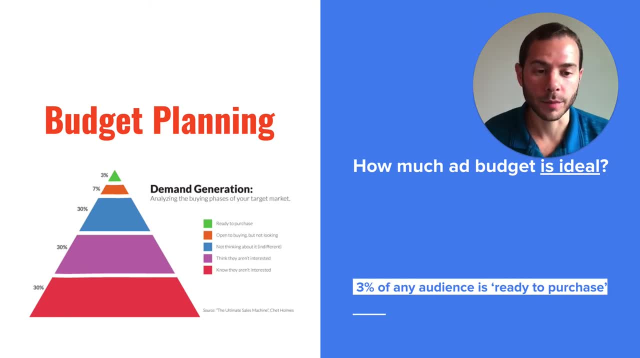 the levels of awareness and where people are in the average market. The main thing to pull out of it, you know, in the average audience, about 3% of people are going to be hot and ready to buy. So keep that in mind when you're generating leads coming into your funnel. is that you know? 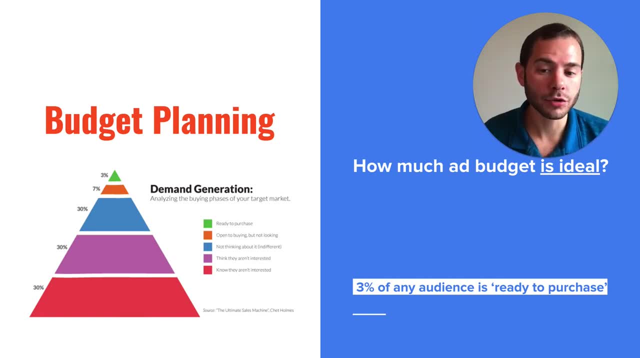 probably 3%, depending on what your offer is and how direct you want to go. Usually it's about 3% to maybe 7%. here are going to be hot and ready to buy And they're going to actively take that next step to booking a call with you or making a purchase on their own. Everyone else after that. 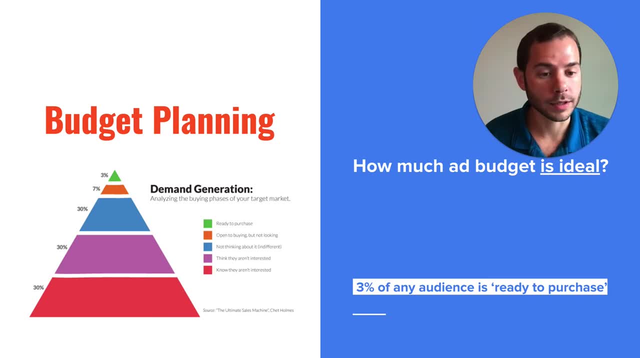 is probably going to need some lead nurturing and follow up. But how this plays into budget is then calculating. how many leads do I need to get a sale, maybe on a monthly basis, And then what's my current cost per lead or cost per conversion, And then what's my close rate on cold traffic. 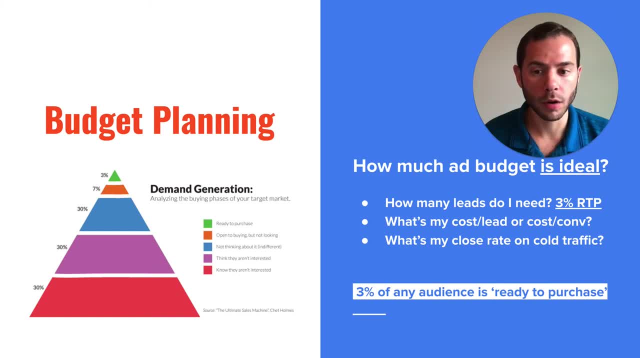 If you've been using referrals mostly before you know your close rate of referrals is going to be a lot different than cold traffic. Cold traffic are people that have never heard about you before. probably need a lot more education and nurturing to have the trust and to have enough information. 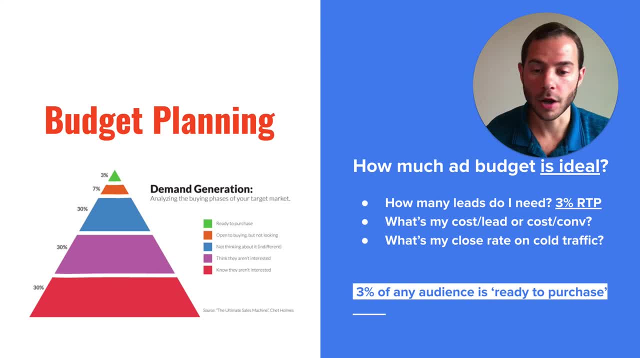 to be able to take that next step and to purchase from you. So keep in mind when you're calculating these: this is going to determine what your overall budget is. You know you'll want to set up an equation to say: if I want one sale a month, how many leads does that mean I need? 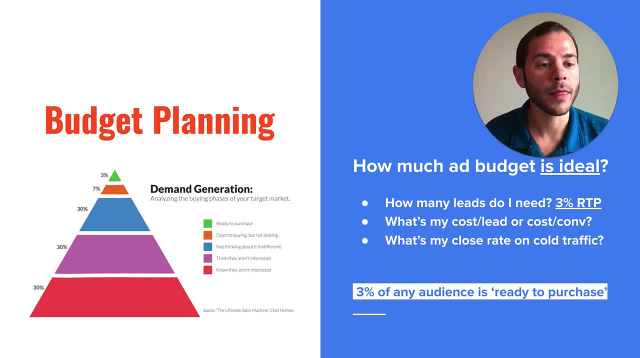 What's my current cost per lead And then what's my current close rate. that'll determine your monthly budget. So usually we say, you know. back in the last slide I said most people start with about 3000 in their first month ad spend And then we see that teams that have sustainable success. 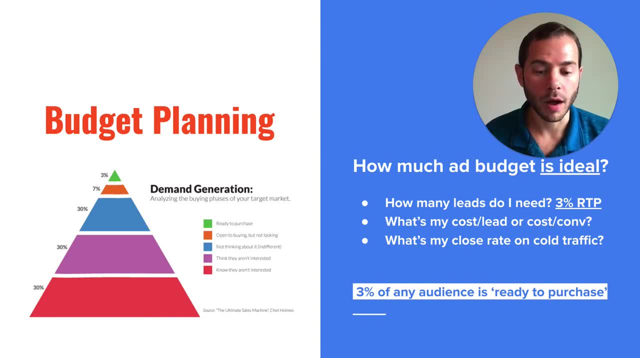 are usually at at or above the 5,000 per month ad spend level And again, that's for targeting middle level people in the U? S. if you're outside the U? S, your budget can be lower than that because clicks are cheaper than that. If you're targeting lower level people, it might be also lower than. 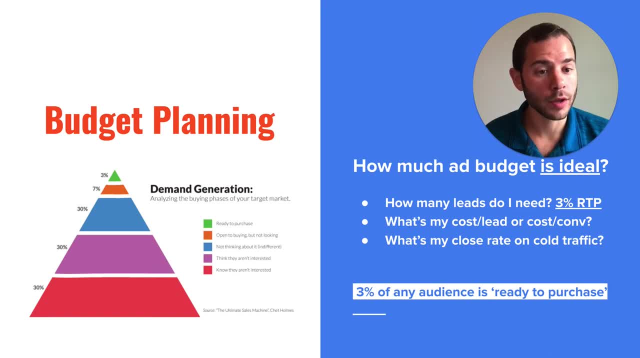 that because clicks will be cheaper. If you are targeting CXO or owners only, your budget might need to be more than that. So you know kind of where that calculates. in the broader spectrum of who's a good fit for LinkedIn, We see that offers that are a best fit or companies that are best fit. 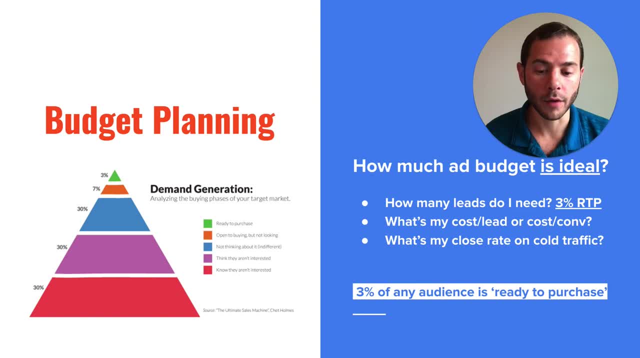 are ones that have a LTV lifetime value of their customer of over 15,000.. So you know if you're paying. we know that LinkedIn is an expensive platform. If you're paying a lot to generate these leads, what is the, what is the revenue you're going to need to make? 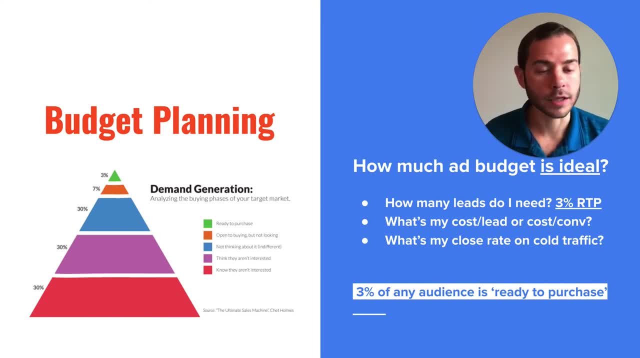 off those people so that the ROI makes sense. And we just see, that's above 15 K. if you're lower than that and your sales process is really honed in, then it can work. But we see, if you're over 15 K. 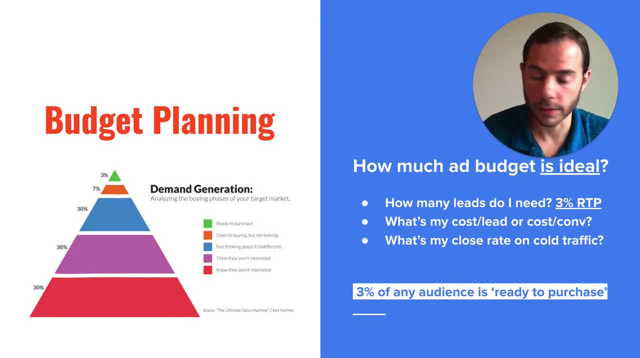 then it's like: okay, I'm pretty sure this is going to work for me. And then the second part of that is having your sales process in place. Cause again: if you're paying- paying LinkedIn prices to generate leads and traffic, you want to have your sales process in place, So you're maximizing those leads coming into your 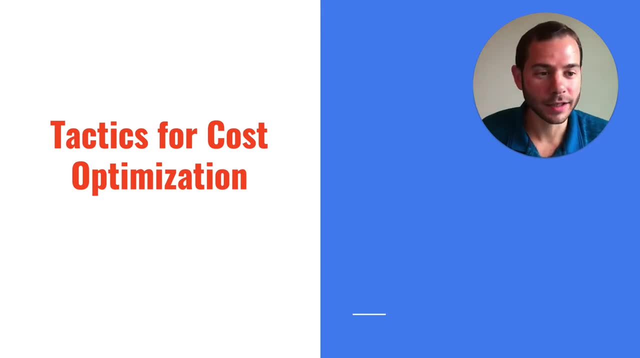 funnel. All right, Now for some fun tactics, for optimizations and like: how do we take this another step further and get even better performance out of this? While there are several things that we'll walk through as we're optimizing a campaign, maybe several different experiments that we'll try- 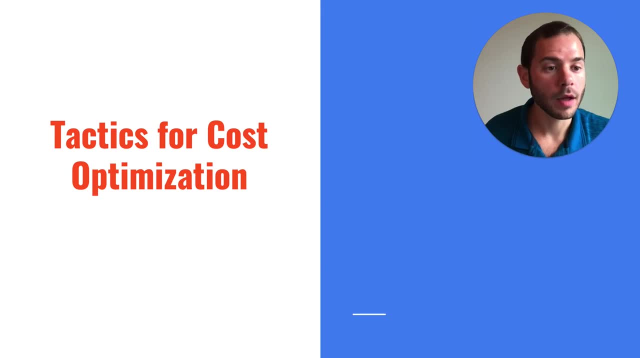 And the first one is what we talked about: manual bidding. Most you know, when you set up a new campaign, by default campaign manager is going to select automated bidding. flip that over to manual bidding- at least a start, and then set. 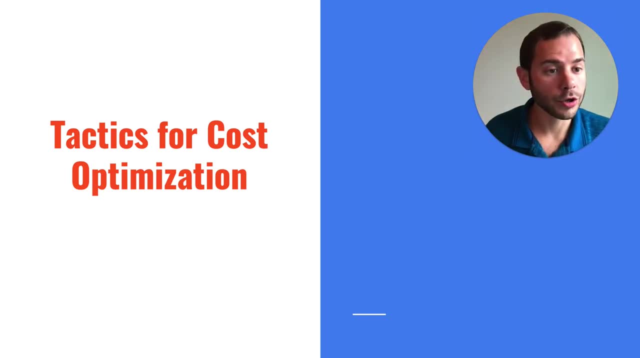 Your own manual bids. Number two is to lower your bids. So LinkedIn is going to give you a default price and they're going to tell you an average range. If your budget is, if you're starting and trying to get the best cost out of your campaign, start by setting that bid as low as possible. 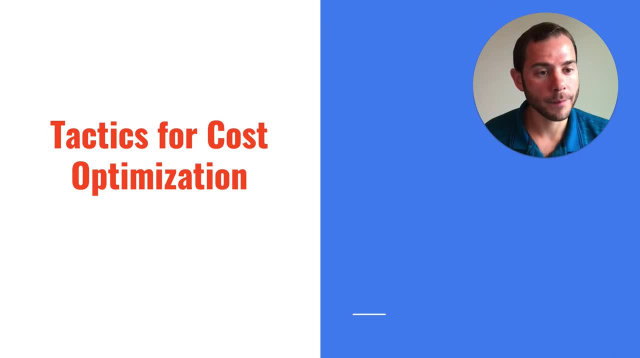 find what the real floor is and maybe start about 20% above that And then you know if you're not getting many impressions, incrementally increase that until you find the sweet spot for your audience. It is a balance between, you know, budget and bid and 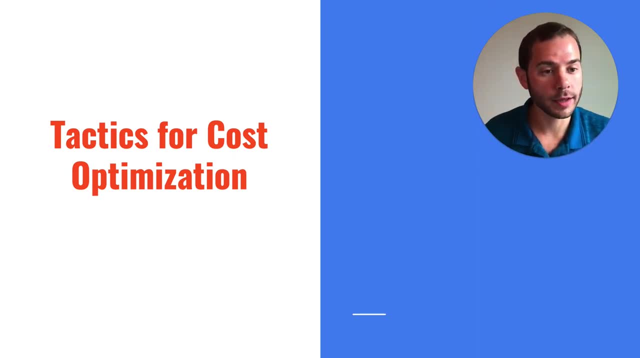 your campaign serving. If your bid is too low and you're not reaching your daily budget, then you know that you'll need to increase that a little bit to spend your daily budget. If your budget increases significantly for what your campaign bids are, you will probably need 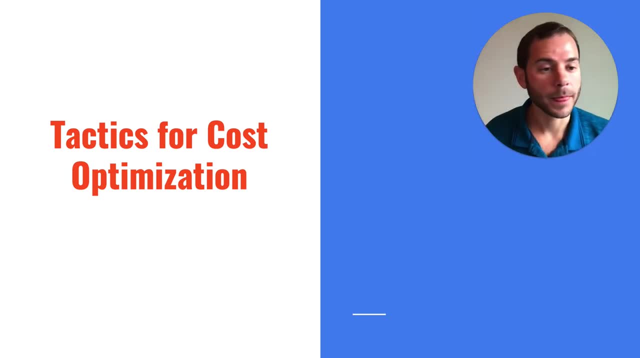 to increase your bid to reach more people to spend your daily budget. So think of it like a balance: The lower your bid, lower bids work for lower daily budgets, but if you have a really high daily budget or monthly budget, then you might need to increase your bid to reach more people. Number three is: 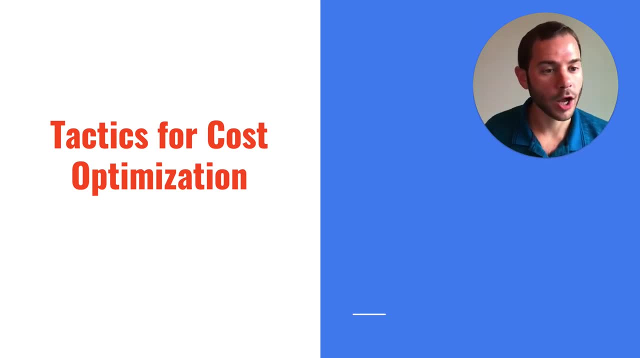 to get creative. So we see campaigns can tend to slow down over time, maybe if that creative starts to fatigue or people are just less interested. maybe the low-hanging fruits already converted. So LinkedIn, LinkedIn's algorithm evaluates your campaign and it's usually based on the click-through. 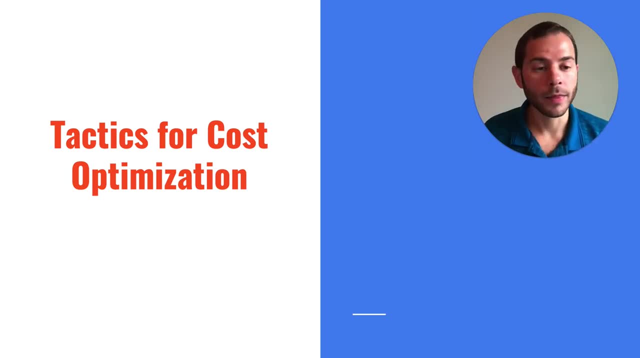 rate of your ads. Sure ads can get reported and other things, but the main way that they evaluate your campaign is through click-through rates. If your campaign click-through rate is low, above that average that I showed you on the first page, if you're below 0.48, then 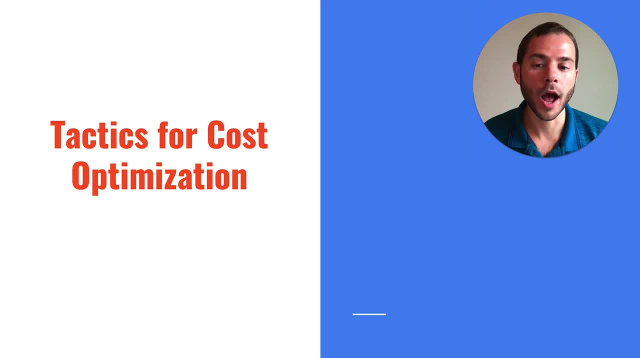 LinkedIn's like this campaign isn't as quality as another advertiser out there. I'm going to prefer letting the other good advertiser reach my audience. So if your CTRs are too low, you will get a lot less impressions, and then you might. 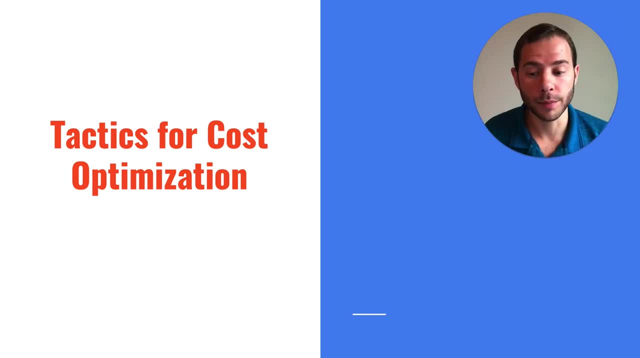 think you need to increase your and then you will need to increase your bids to reach more people. So often we'll see if we can increase CTRs on a campaign and on ads, then often our costs and our bids get cheaper, which improves our cost per conversion and cost per lead. 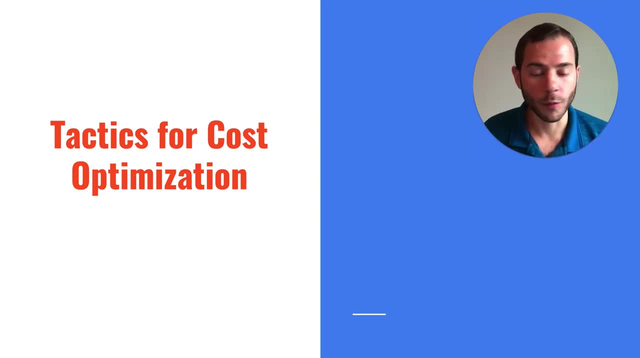 Number four is narrowing your audience. So one mistake we see a lot of people make is maybe they've tried Facebook ads or Google Display and they're moving over to LinkedIn ads here and they're taking a very big audience that they had on Facebook and just porting that over and making some similar guesses. 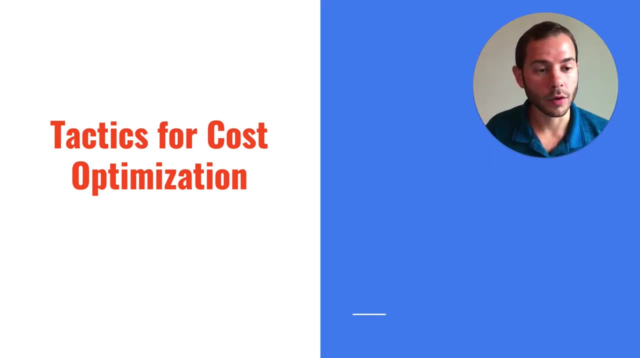 on LinkedIn. But on LinkedIn because if you follow these recommendations, you're usually paying for every click to start. You only want to get Really targeted clicks. So we see most people. the problem they have is they have a very big audience and then 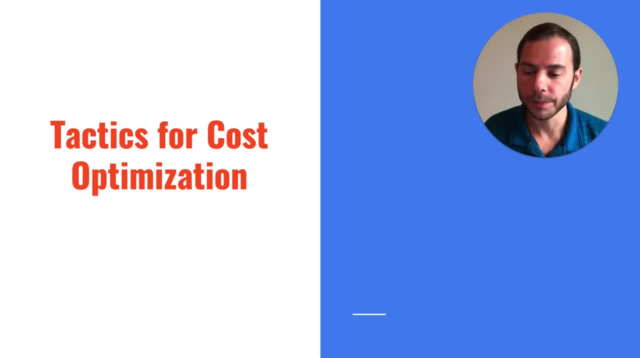 not necessarily everyone in the audience is interested or really a candidate. So we find that, to start, you want to narrow your audience into the absolute People who are absolutely most likely to be interested, And you can do that by layering in skills and groups and interest targeting to make 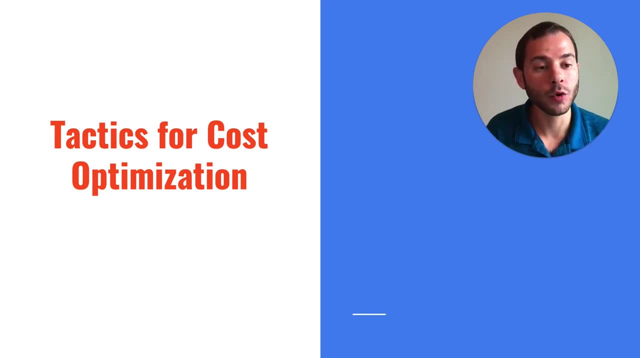 sure, at the beginning especially, you're very honed in on who is going to be most interested in this offer. That will then increase your CTRs, increase your conversion rates and they improve your costs. So once you've found your kind of sweet spot- audience- then the next tip here is to go. 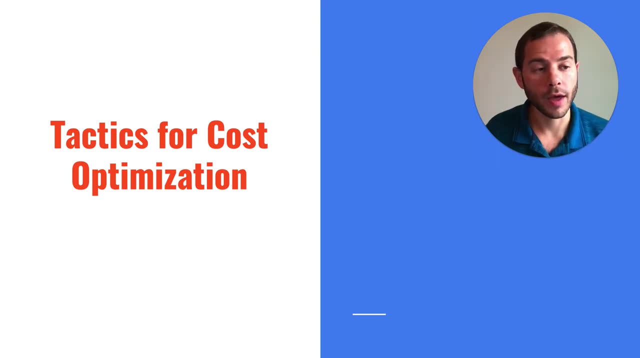 and expand your audience. So if you have a very small audience then it's going to be more expensive to reach those people. In general, the bigger your audience, the cheaper, The more cheaper people are going to be in that audience. If you have a very small audience, you're forcing the algorithm to go essentially overpay.